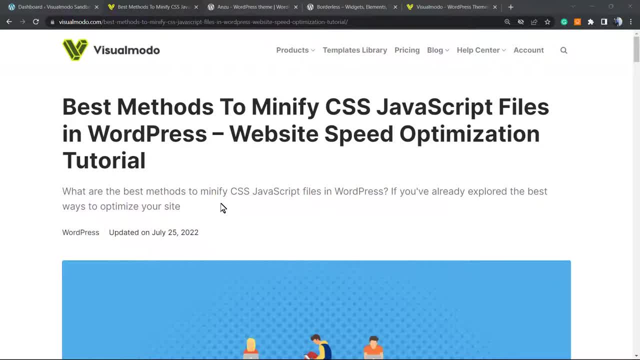 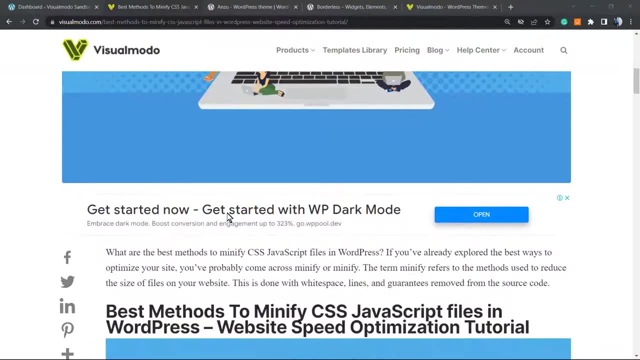 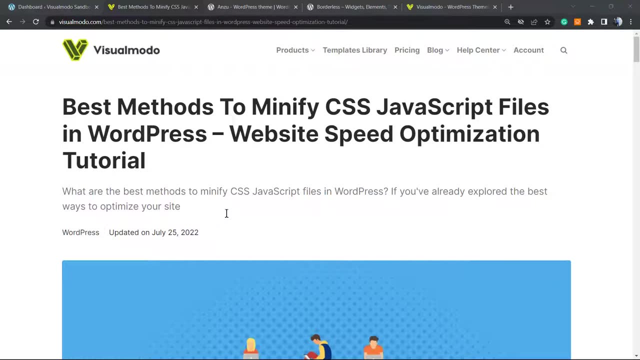 explain how to do this in a simple way, for free, without coding. okay, So no need to pay, no need to code and no need to worry. simple as it is, But before take a moment to hit the subscribe button, like this video and share this content with a friend of yours. 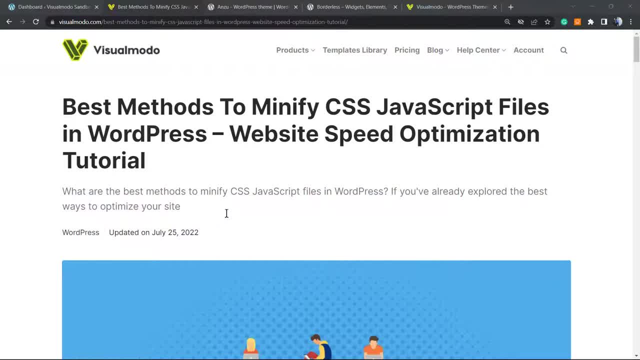 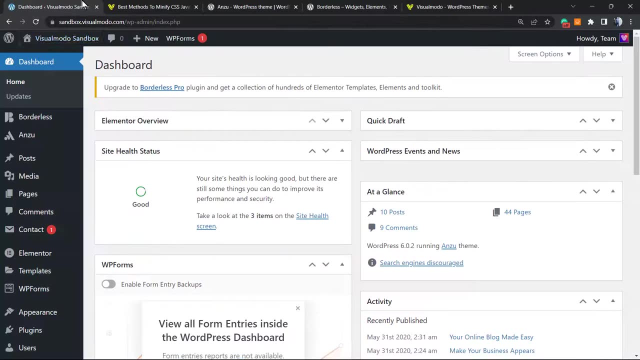 You have no idea how much it help us, help the channel and the fact that we bring daily videos about WordPress, SEO, commerce, sales and many more topics in order to have an amazing site, And we will help you by any means as well. But let's go to the WordPress dashboard. that 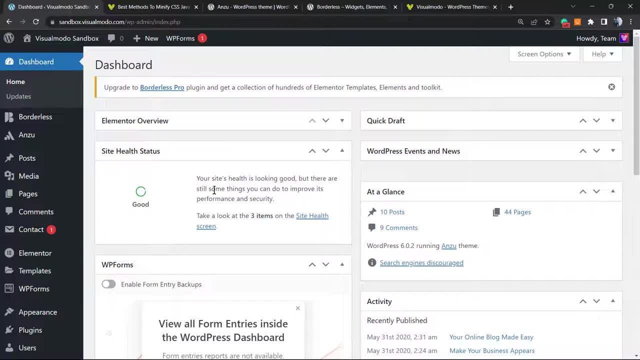 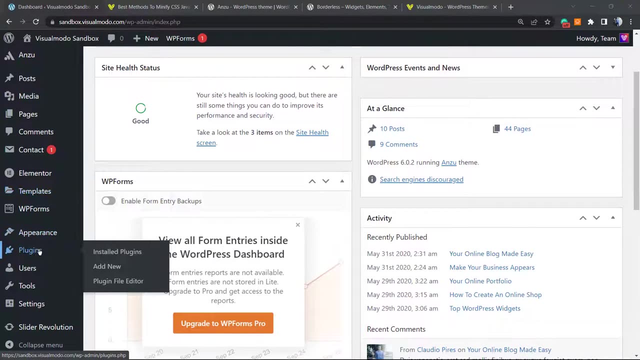 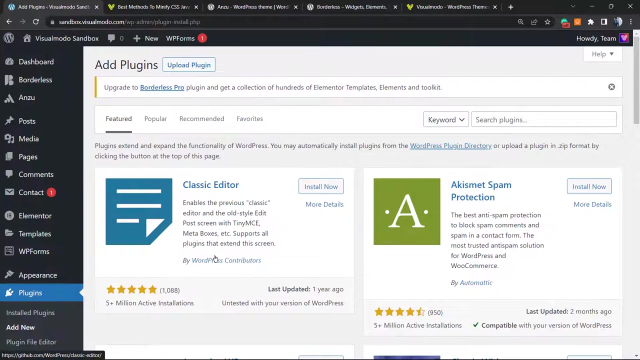 is the place where I normally likes to start all my videos, because it's equal for everyone. So go to our WordPress dashboard, okay, And from the WordPress dashboard, navigate to the section called plugins. okay, And go to add new. Just before anything, note if you. 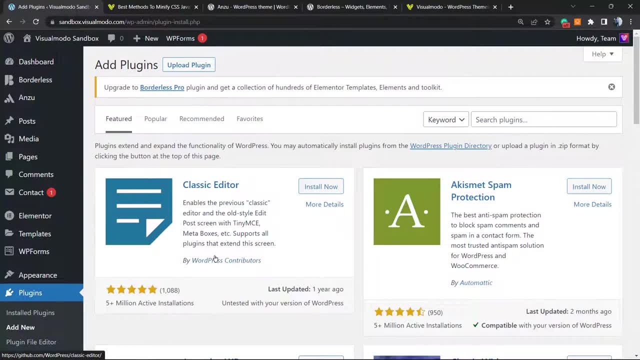 are using WP Rocket plugin. no need to do this. You have an option on WP Rocket. I'm gonna write another video explaining how to do this using WP Rocket. But if you did not want to pay for WP Rocket once it's a premium only plugin, you have a free method to do. 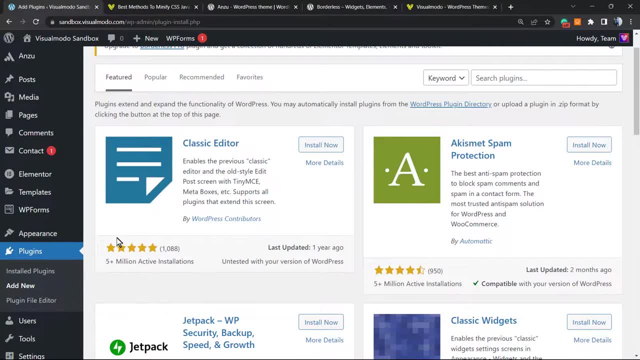 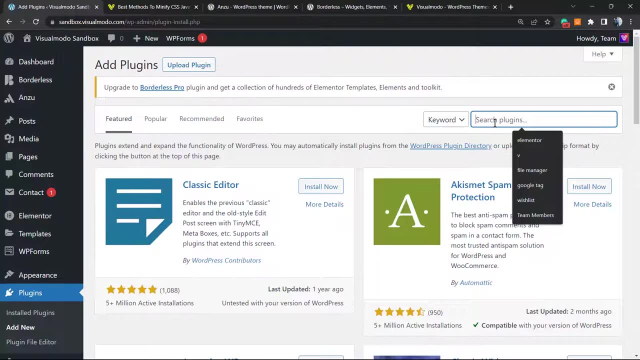 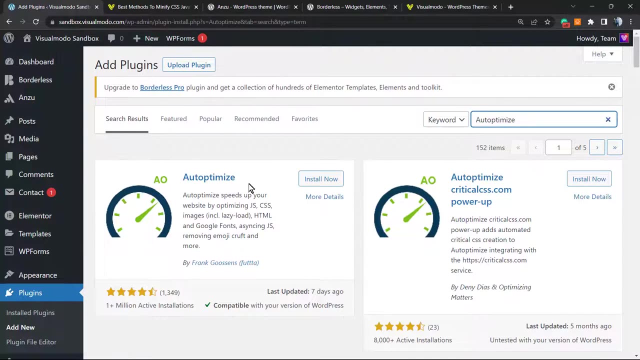 this without investment. okay, And this is the one we're gonna teach. So WordPress dashboard, left sidebar of menus- plugins- add new. and into the search field at the upper right corner we're gonna type auto optimize. What is this? This is an amazing plugin in order to make 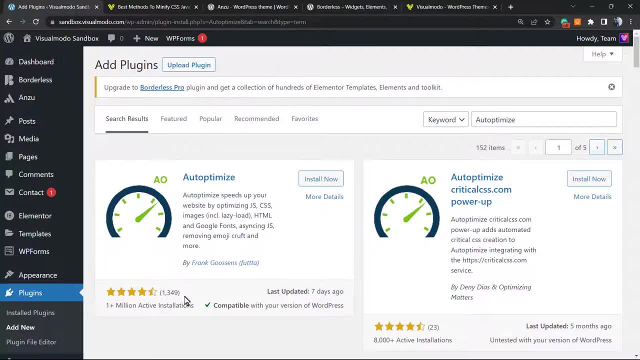 your site loads faster And, as you can see, it's very well known. It's active in one million websites. It's compatible, has been updated seven days ago. This is a very important part, okay, So click on install now And, Frank, if you are watching this video, thank you. 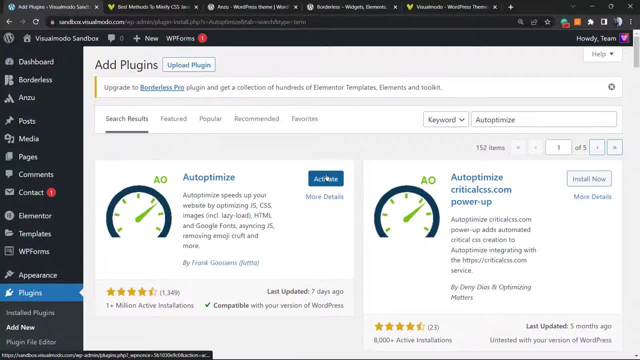 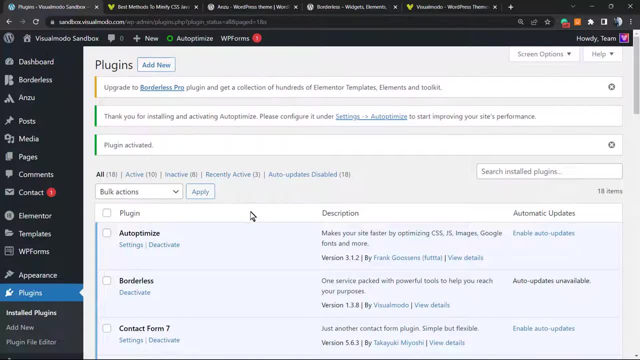 so much for a great plugin. After installation: complete click on this activate button. okay, It's gonna start. Okay, so now we're gonna go to our WordPress dashboard and we're gonna redirect you to the WordPress plugins list page, a list where you can see all of your 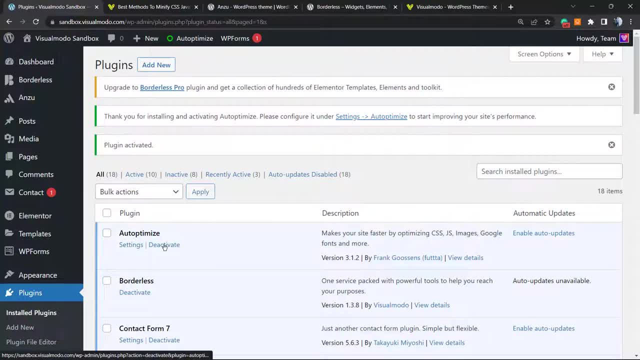 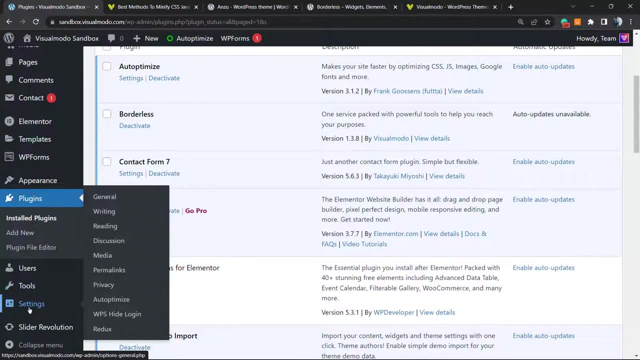 plugins And from this list we can access the WordPress settings already activated- okay. But in the case that I want to find a plugin, it's under settings next to tools. okay, On your WordPress left sidebar, Next to privacy, you have the auto optimize And 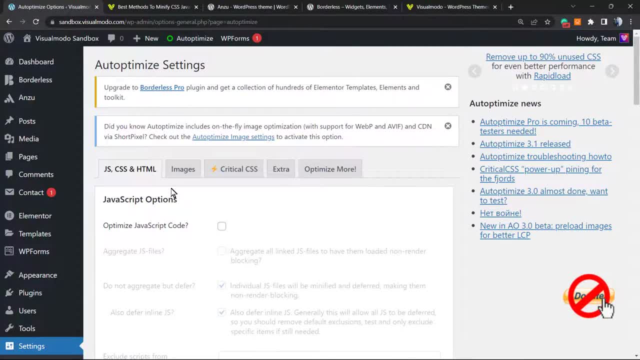 here is the guide. Can you see how simple it is to activate This plugin? have a lot of options, okay, Have nice things in order to optimize your website for speed, But the very first one that you're gonna be activating is this one. 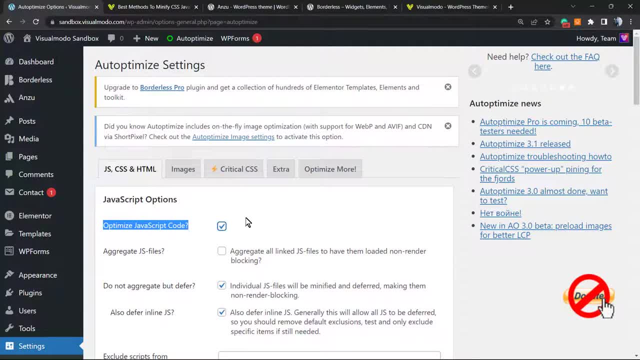 optimize JavaScript code. okay, Active this. aggregate JS files. This is good, okay, But normally it changes according to the plugins that you are using, to the code style of your theme, of your plugins, of your content. Next, you can activate in the case that you want, whoever. it might generate some issues. 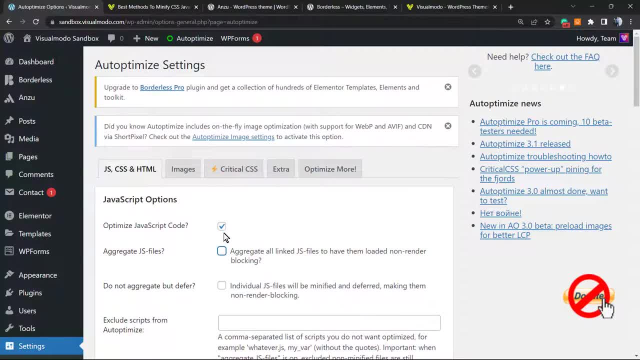 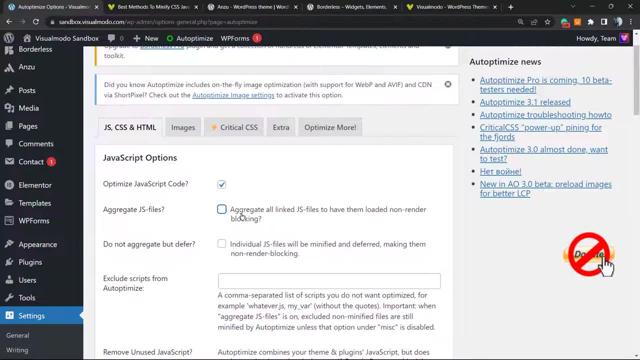 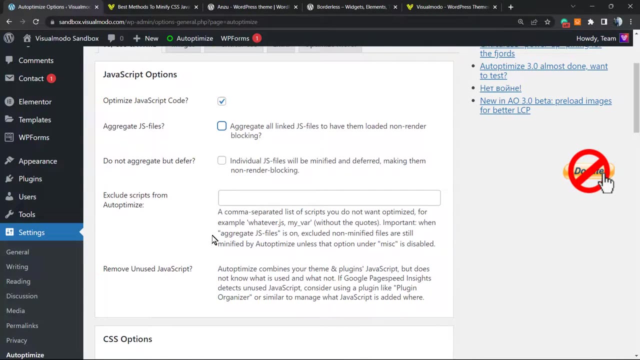 on your site. okay, So as soon as you click on it, you can just update the settings. okay, So leave other blanks. You have other things. For example, you can exclude some scripts in the case that you want. You can remove unused script. okay, And we have the CSS options. 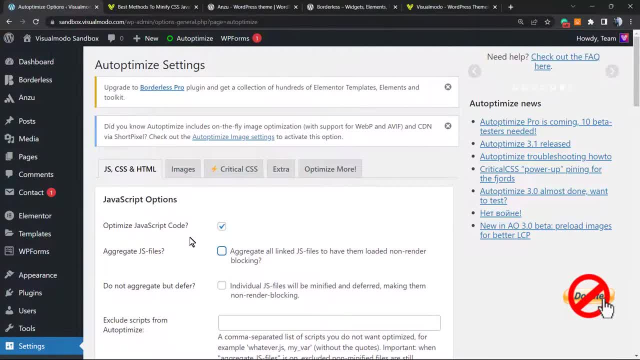 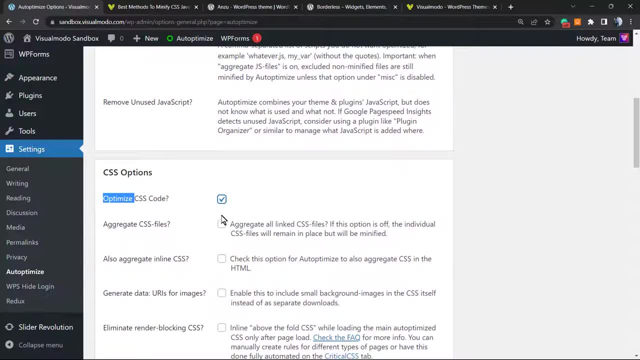 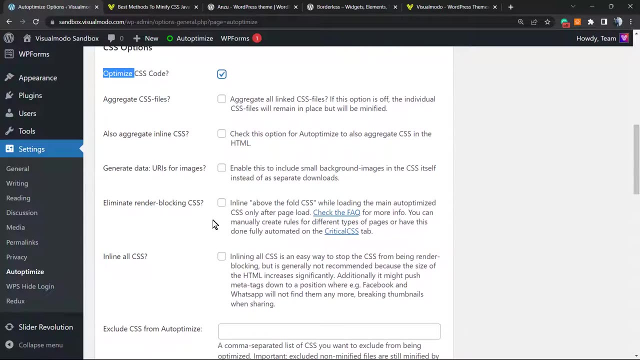 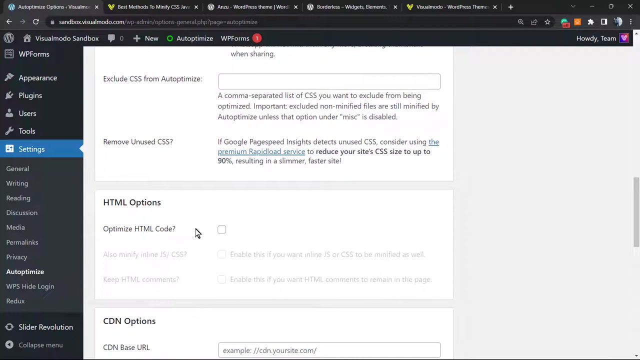 right here. So we already optimized it, or JavaScript code, And after this, optimize CSS, Optimize HTML code. This is another good part of this plugin. okay, This is a great part of the plugin. Okay, You can actually break your site. okay, So activate, test the front page of your site. 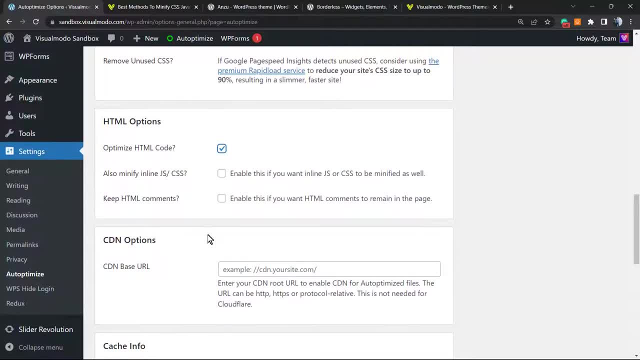 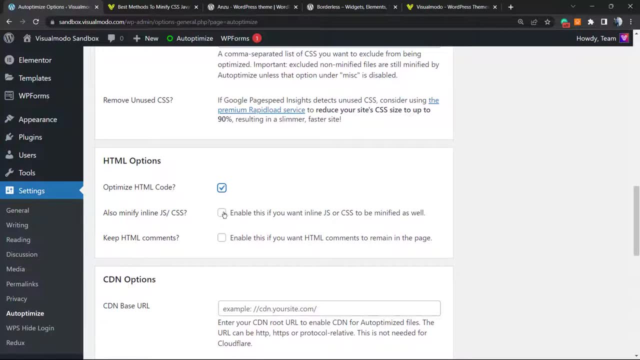 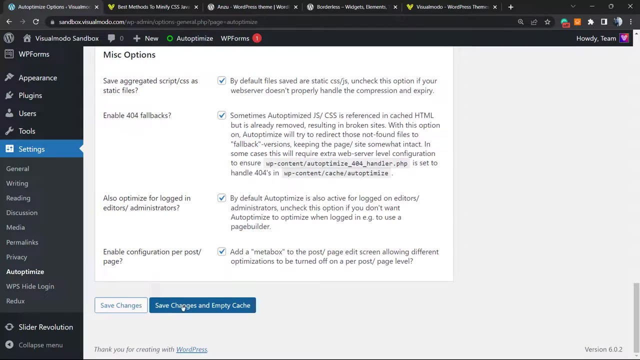 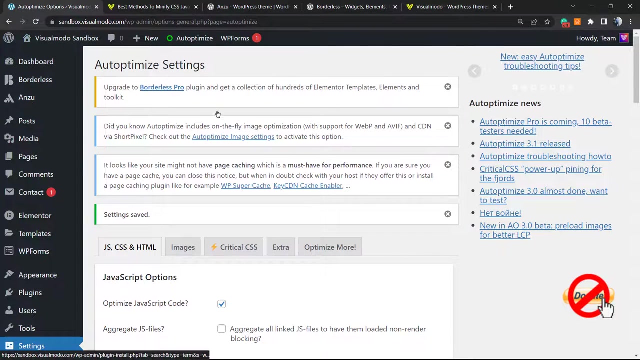 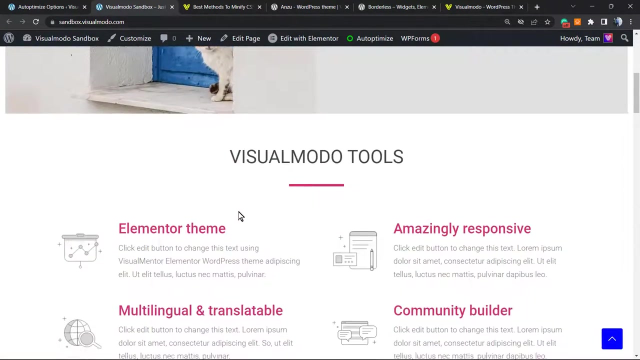 and review if it's working for you or not. okay, As you can check, we have lots of options. Let me save changes and empty cache. okay, Changes are saved. Let's review our website to check if anything breaks. All seems good. 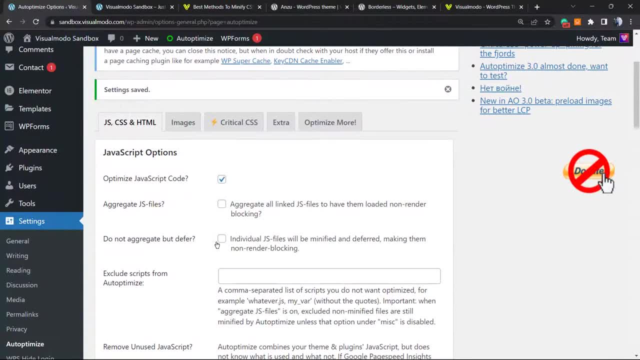 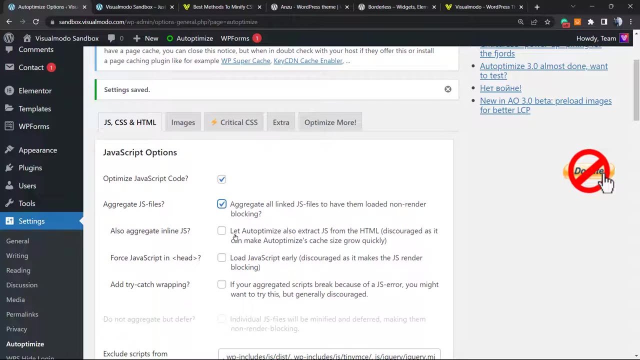 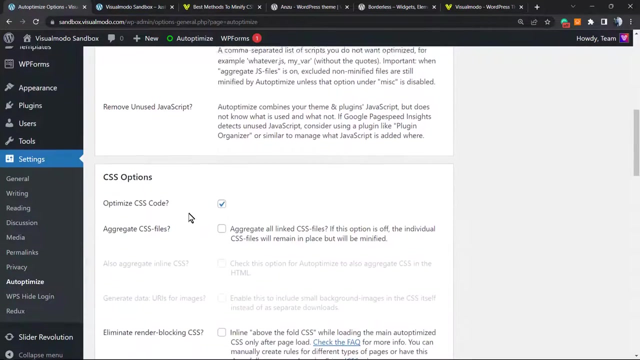 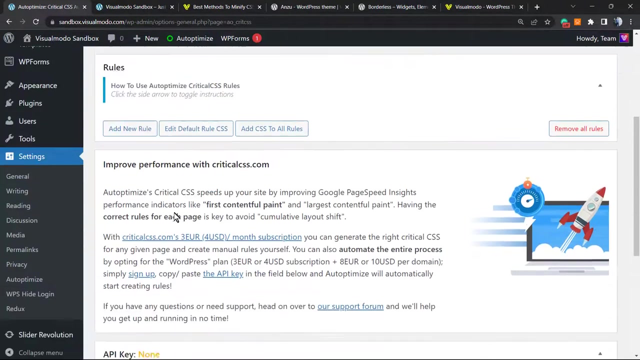 Now we already have the minified versions of the files. Can we aggregate the files? Of course we can. Okay, Okay, And we're already good to go. They have other things, for example the critical CSS, in the case that you want. 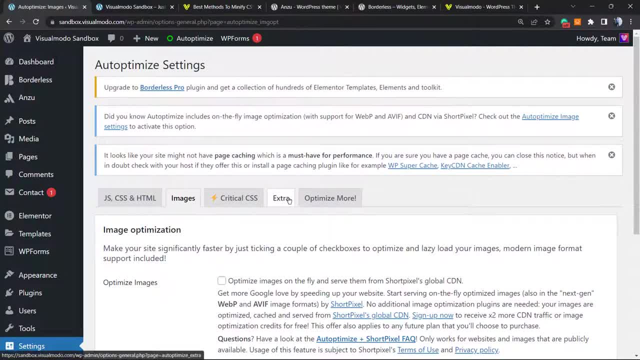 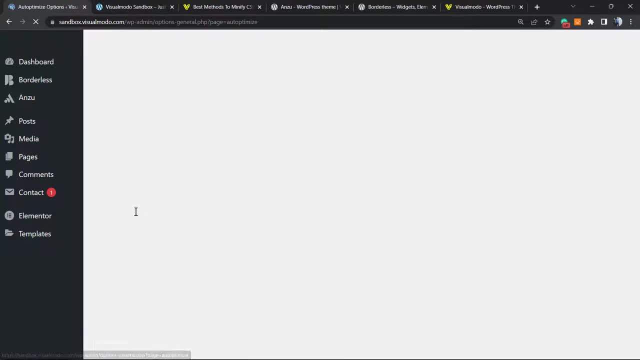 You have the image optimization, in the case that you want. You have some extra models, in the case that you want. There's a lot of things to explore on this plugin, But the most important part are just these simple settings. So click right here. 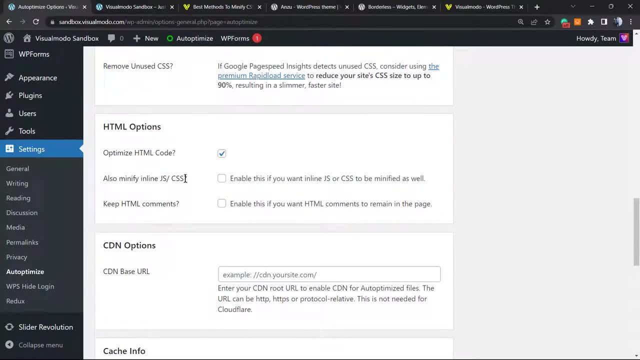 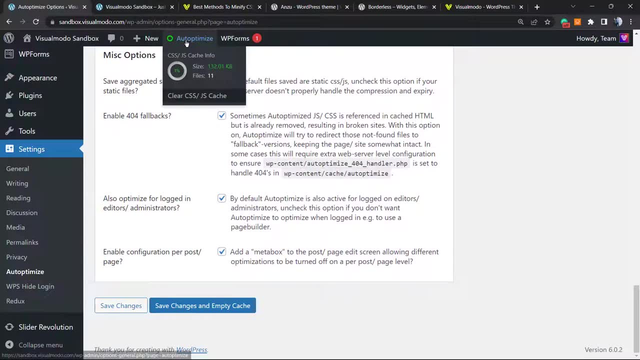 Okay, click right here. you can also click right here, and you are good to go. the file is going to be minified. okay, click on save, change, clear the cache, and you are good to go. and here is the plugin working. as you can see, there's a new bottom on the top of your wordpress. 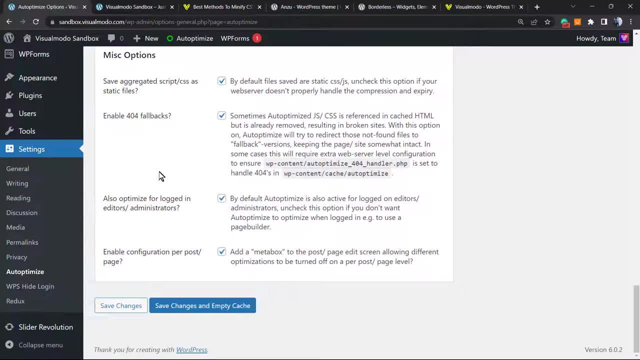 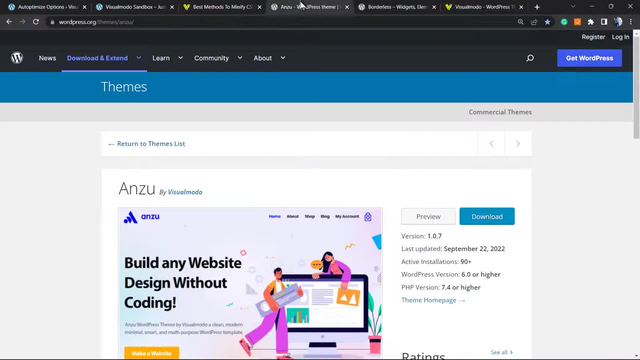 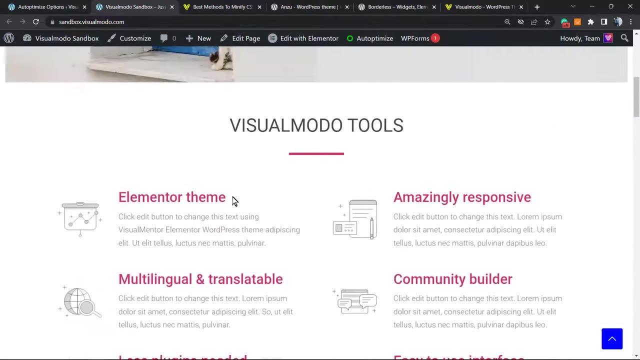 that appears for the login users, and it is. i hope you guys enjoyed this video. feel free to use the comment section below in the case that you have any question, and don't forget to check out our enzoo free wordpress team to install this amazing wordpress team and create a website like this one. 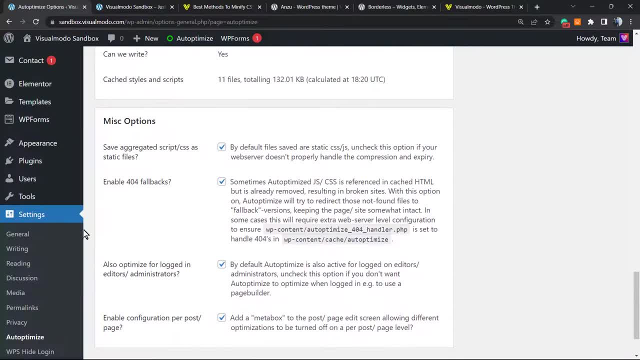 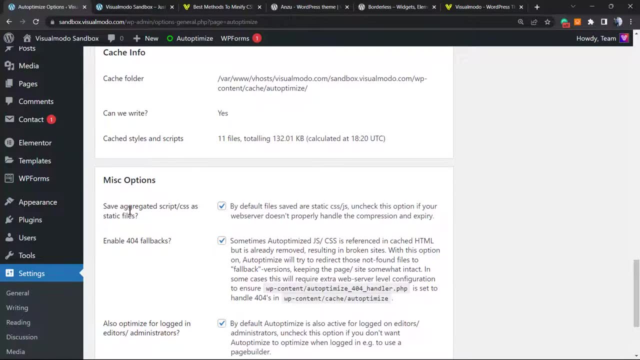 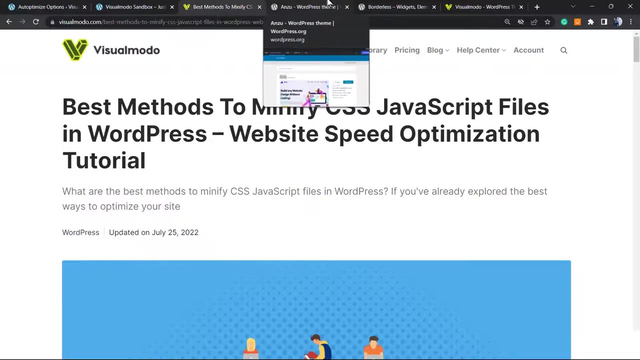 or a fully customizable site. go to our wordpress dashboard appearance themes. search for our enzoo and install. it's completely free and have amazing features, okay. moreover, in the case there are needs of enlarging the amount of settings that our page builder have, go to our website dashboard plugins. 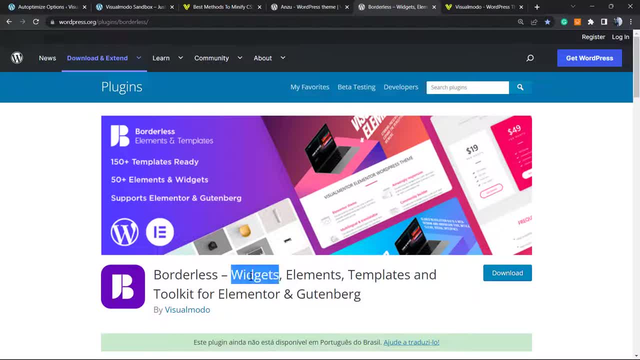 add new and search for enzoo free wordpress team to install this amazing wordpress team, our borderless wordpress plugin, because it gonna brings you widgets, elements, templates, tools and many more things good for your wordpress website or landing page. and, as a final notice in the case, 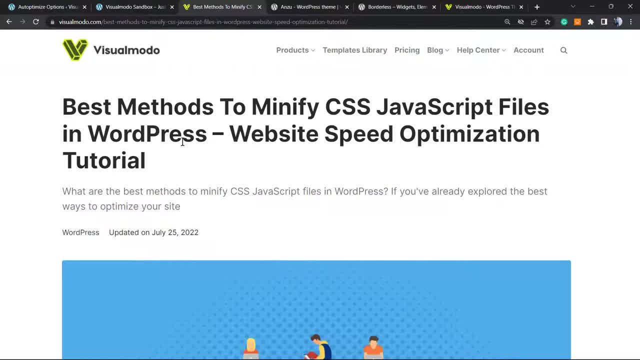 that you prefer more details, would like to know more options in order to minify css and javascript files on your wordpress? go to our blog on visualmodelcom. give you our blog and check our full tutorial right here. okay, and finally, in the case that i need,